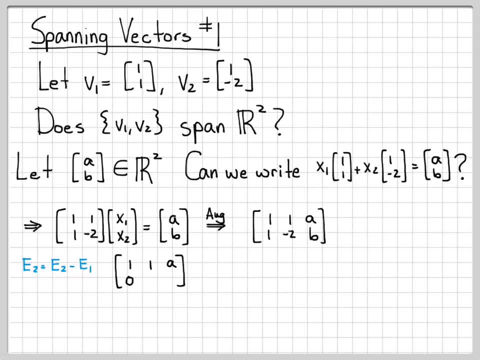 here, because 1 minus 1 is 0. And negative 2 minus a negative 1 is a negative 3. And then b minus a is b minus a. So there we have that. And then if I let e2 equal a negative 1, third e2, multiply every. 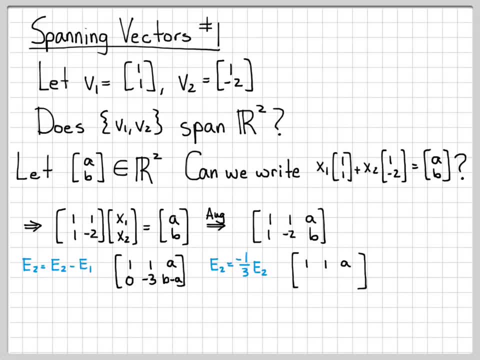 quantity by a negative 1. third. equation 1 will be unchanged. 0 times a. third is still a third. A negative 3 times a negative 1. third is 1.. And then we have a minus b or b minus a times a negative 1, third. The sign changes so that turns into a minus b over 3.. And then 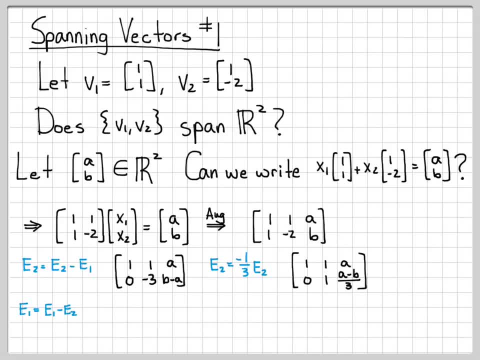 finally, let's go ahead and let e1, equation 1, equal equation 2 minus a negative 1.. And then let's go ahead and try to get a 0 right there. So if we do this, equation 2 remains. 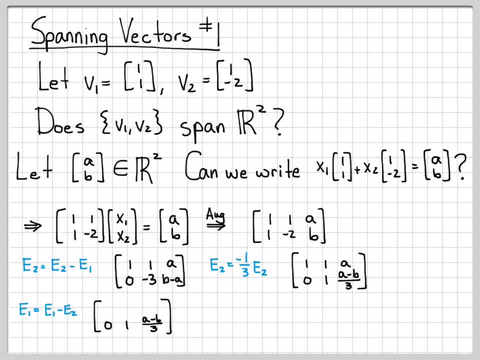 unchanged. But equation 1 in the first entry will be: 1 minus 0 is 1.. 1 minus 1 is 0.. And then a minus the quantity, a minus b over 3.. So I have done a few row operations to manipulate this augmented matrix. And now, by looking, 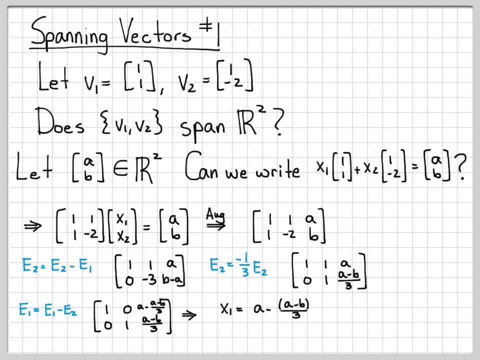 at this, it's very easy to see that x1 is equal to a times the quantity a minus b over 3. And x2 is equal to a minus b over 3. So there I've been able to find numbers x1 and x2 that 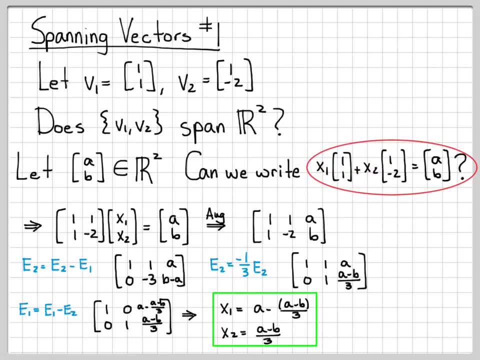 make this equation true for any value of ab that I want to choose. So, remember, we've chosen this arbitrary element from r2.. And I've been able to find these coefficients that make this equation true for any arbitrary element from r2.. So, yes, these vectors do. 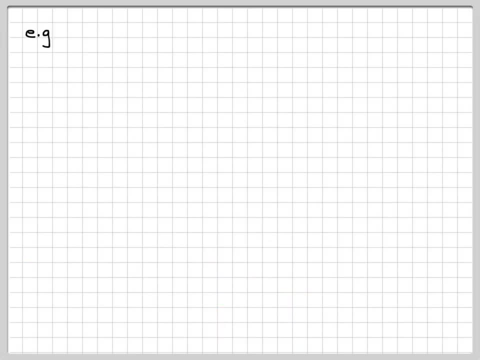 span r2.. OK, So let's continue with just a little example here. So just to make it concrete, we did it generally, But as a for example, if I chose the vector 4 negative 2, I could go ahead and compute what x1 and x2 are based on the solution we just found. x1 would be 4 minus. 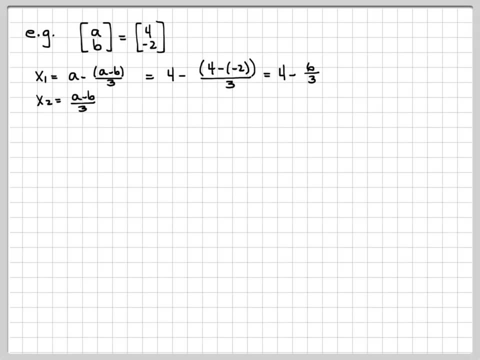 the quantity 4 minus a minus 2 over 3,, which is 4 minus 6 over 3,, which is 4 minus 2,, which is 2.. Similarly, we could compute x2.. It is 4 minus the minus 2 over 3,, which is 6 over.